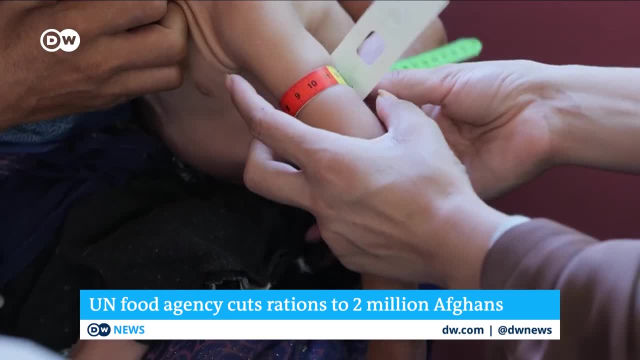 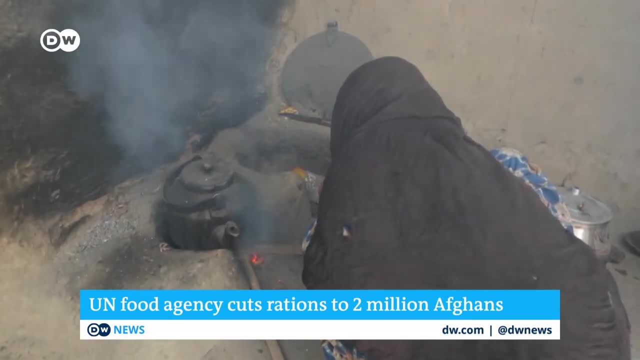 The UN is raising the alarm over shrinking aid to the country, warning of a catastrophe if things don't change. It said the World Food Program now has to choose between the hungry and the starving in a country where most already don't know where they'll get their next meal. 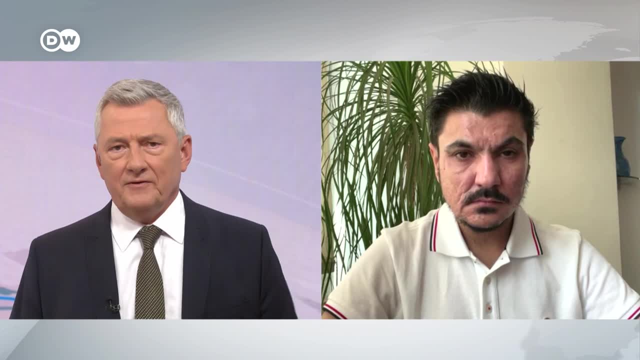 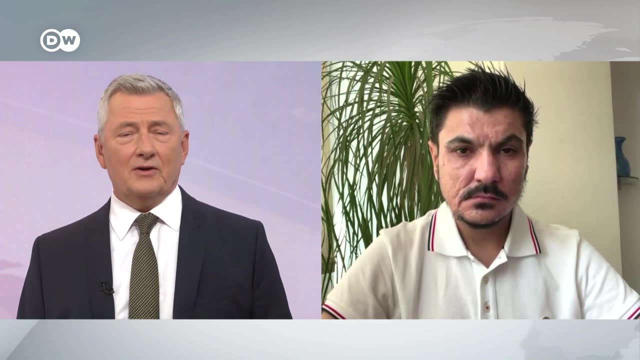 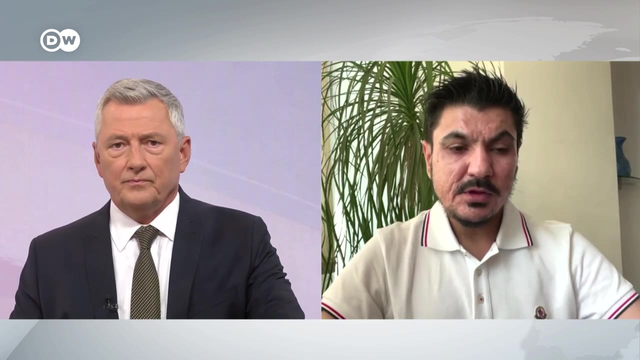 We're joined now from Kabul by Ali Latifi. He's the Asia editor at the New Humanitarian Ali. how bad has the humanitarian situation become for the people in Afghanistan since the Taliban regained control? I mean, you just have to look at the UN statistics. Over the last two years, they've consistently said that something between 18 and more than 20 million people will be in need of some kind of emergency assistance over whatever year we're talking about: 2021, 2022, 2023.. 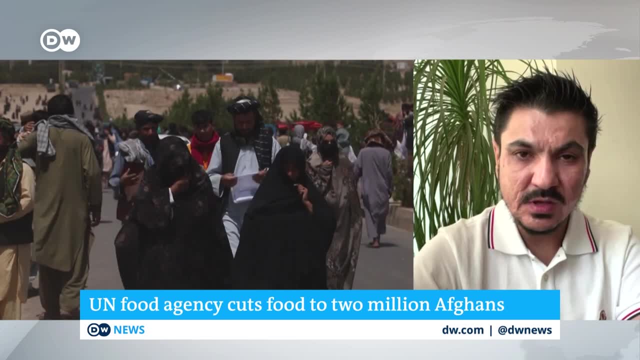 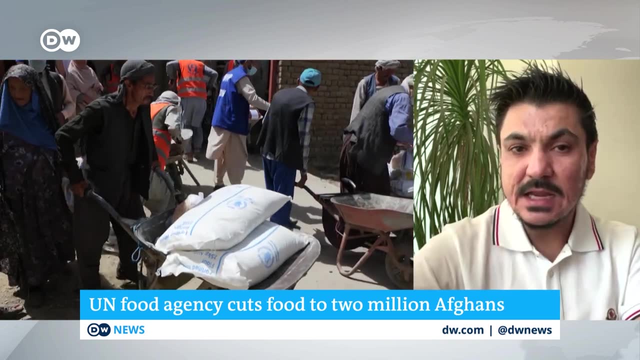 And this year is no different. This year, I think, was estimated around 20 million already. So now you're adding what you're taking away: 2 million more, 10 million more. You're just adding to what it's already called, I think, like the world's largest humanitarian crisis. 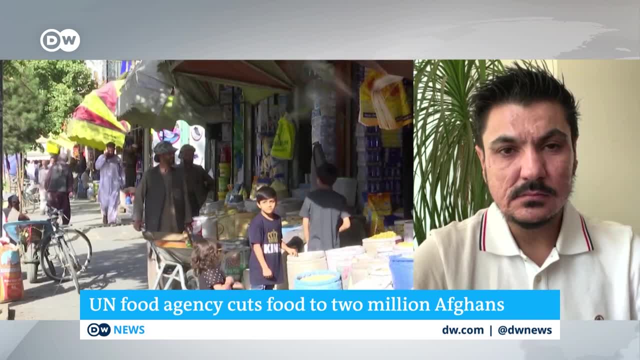 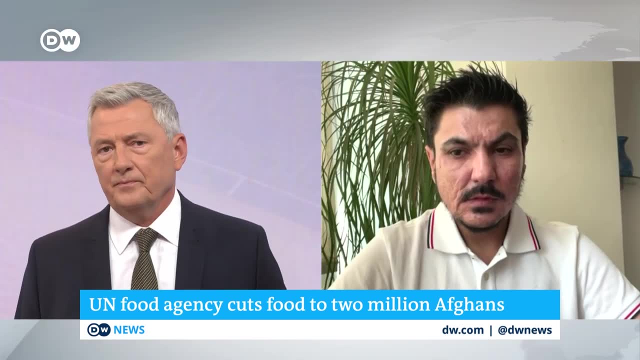 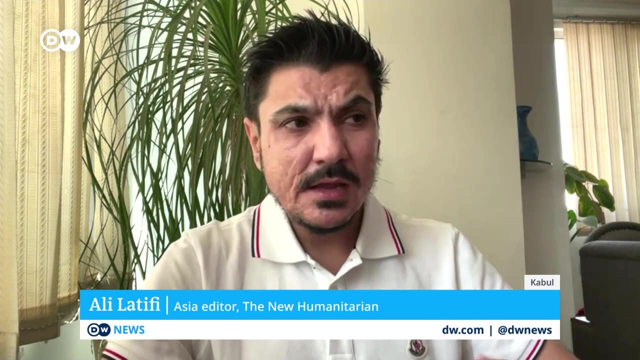 So it's very evident that there's an issue here. Who are the people most affected by the shortage of food? Ali, I mean, you're talking about. you know, very rural people, people who used to be farmers, who were still farmers, who you know had to deal with the devastating effects of, in the last two years, earthquakes, floods. 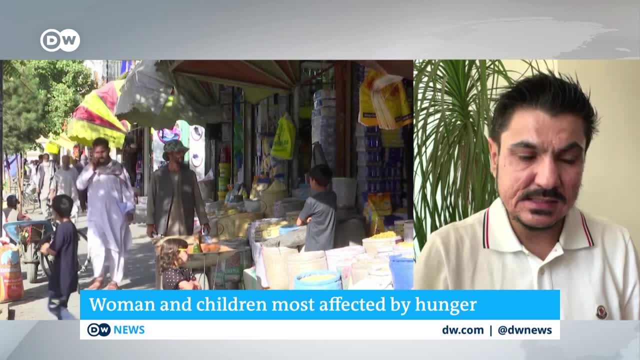 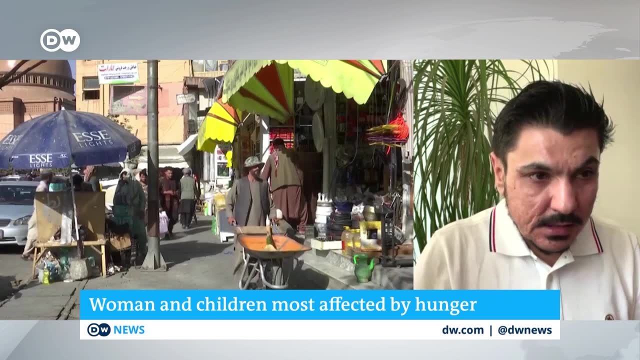 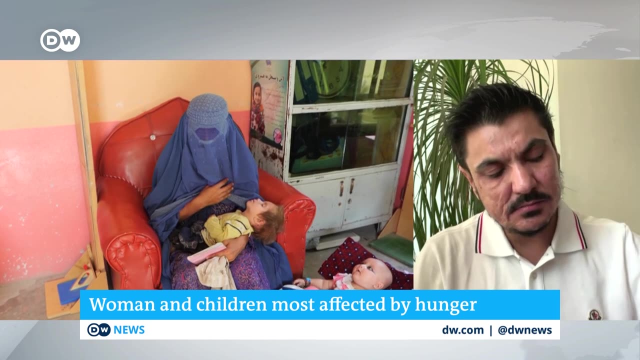 Droughts, who were already essentially living, subsistence living, And then, when the economy overall collapses and, you know, investment lowers, they continue to suffer. They are suffering not only because of natural disasters that are beyond their control. they're also suffering because of economic issues that are also beyond their control. 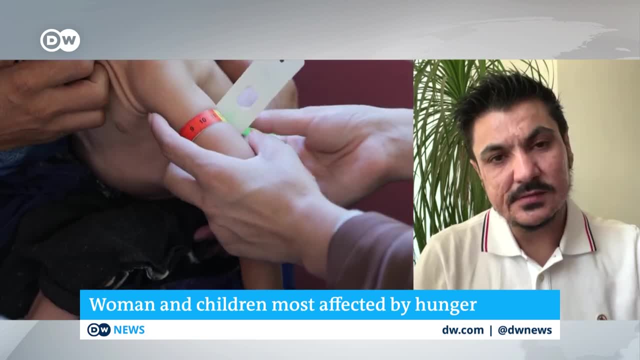 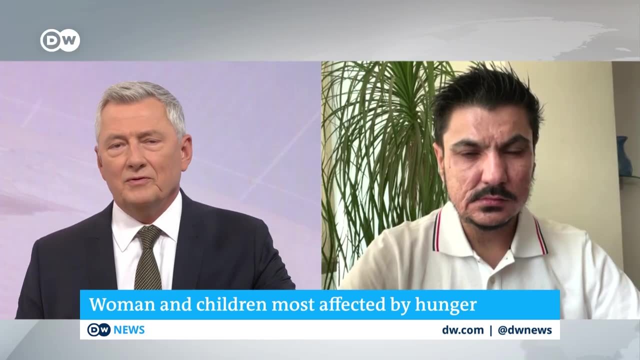 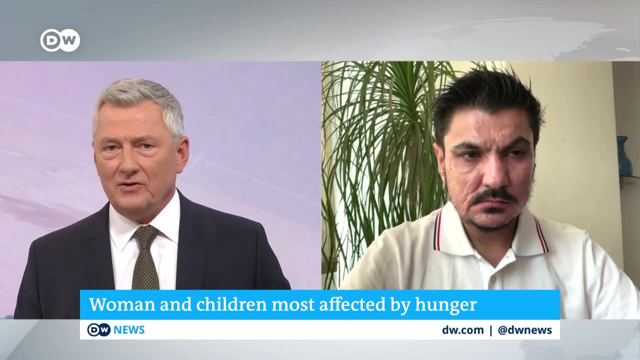 which means that they are finding it more and more difficult to feed themselves and their children. So the people in Afghanistan are not chiefly responsible for what they're facing. it sounds like you're saying Who would you say is chiefly responsible for the humanitarian crisis that we're seeing in Afghanistan today. 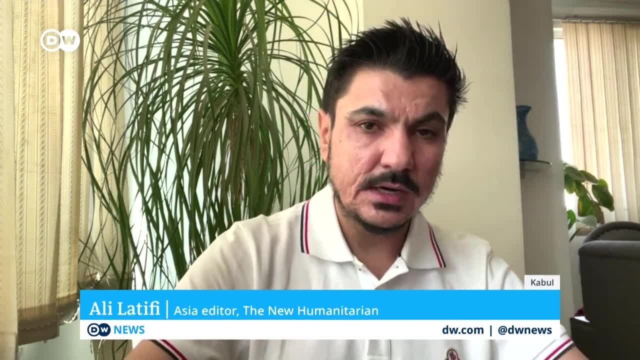 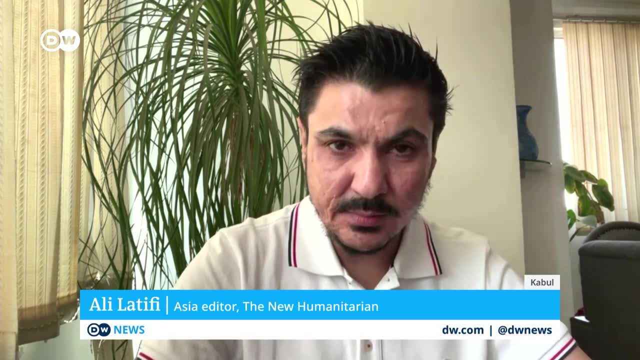 The international community, because you're talking about an economic crisis that was created after the Taliban took over, which the international community knew was going to happen. They knew the Islamic Emirate was coming back into power And immediately they inflicted sanctions, banking restrictions, they withheld assets.